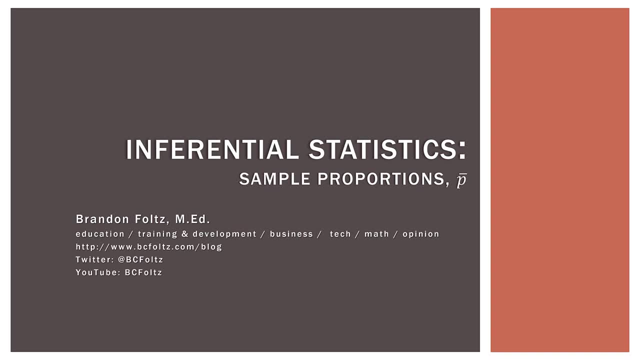 And actually underneath it's very simple. But when we talk about other things like the standard error of the sampling distribution and finding probability intervals, it can get a little bit more complex. But almost everything you're gonna see here goes back to what you saw talking about sample means. 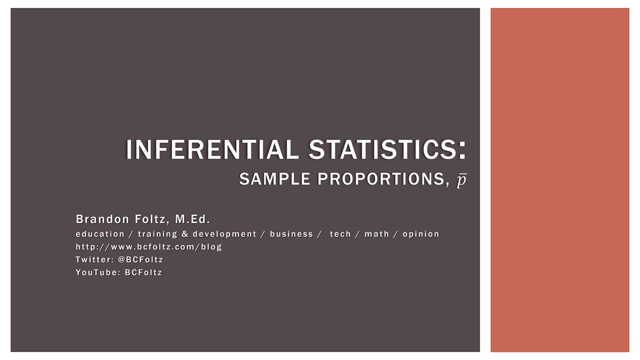 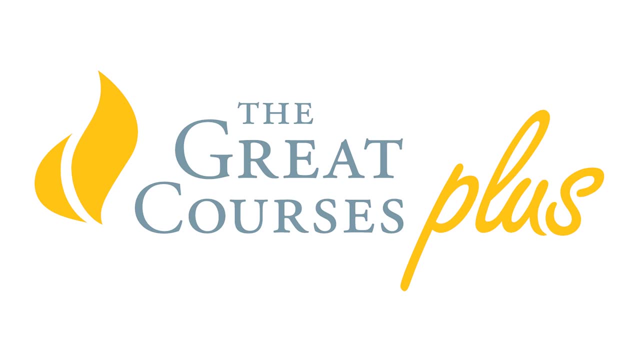 So we're gonna go from sample means to sample proportions, with a few similarities and a few differences. So let's go ahead and get going. So this video is brought to you by the great people at The Great Courses, Plus, Chances are, if you're watching this video in the first place. 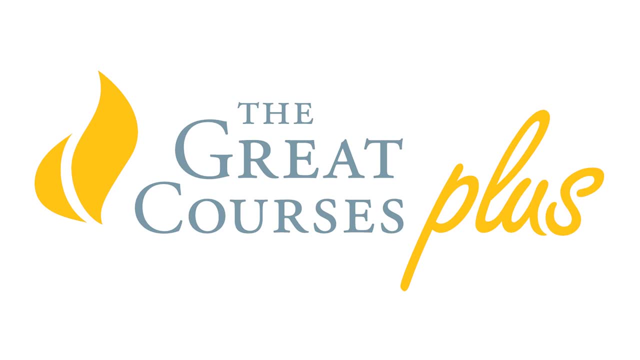 it's because you need to or want to learn something, And there are few better places to learn about anything than The Great Courses. Plus, They have over 11,000 video lectures on almost any topic imaginable, from photography to philosophy, to history, literature to gardening. 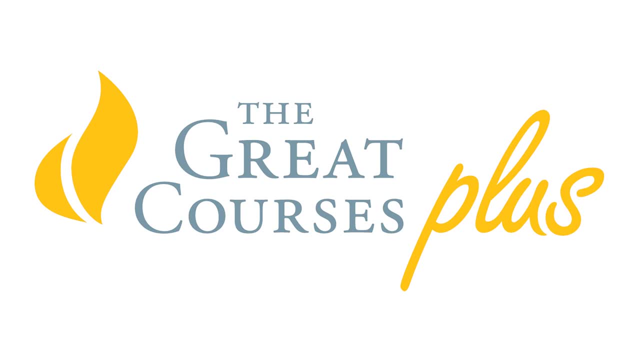 and, yes, of course, math and statistics. And, luckily, The Great Courses Plus are giving my viewers a free trial, So please click on the link in the description below to support this channel and, of course, support The Great Courses Plus. Let's go ahead and get started on our topic. 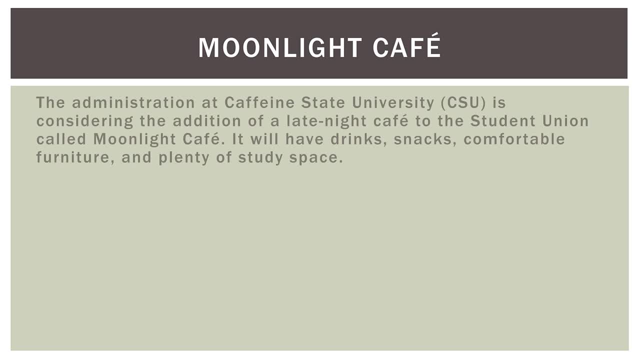 So what's going on at the Moonlight Cafe? The administration at Caffeine State University, or CSU, is considering the addition of a late night cafe to the student union called Moonlight Cafe. It will have drinks, snacks, comfortable furniture. 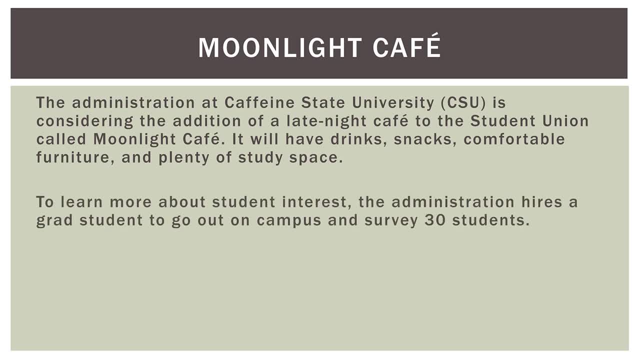 and plenty of study space. To learn more about student interest, the administration hires a grad student to go out on campus and survey 30 students, Yes or no? Would you study at Moonlight Cafe at least once per week? The result of the survey is that 17 out of 30 students 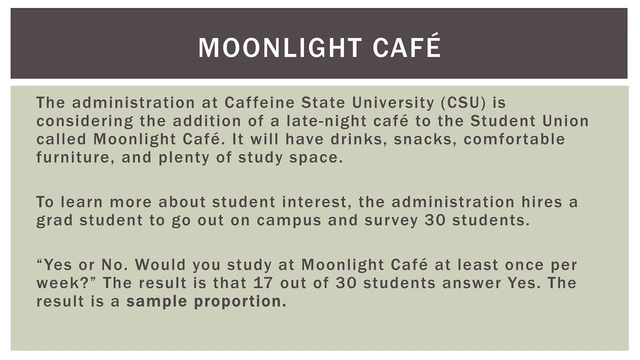 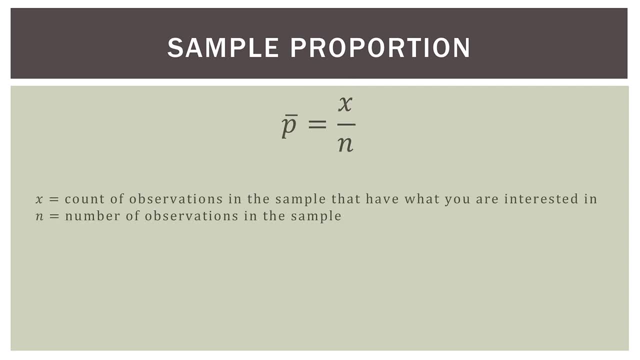 answer yes. So the result is called a sample proportion. Now, mathematically this is a very simple concept. So the sample proportion is represented by p bar. So remember: the sample mean is x bar, The sample proportion is p bar. 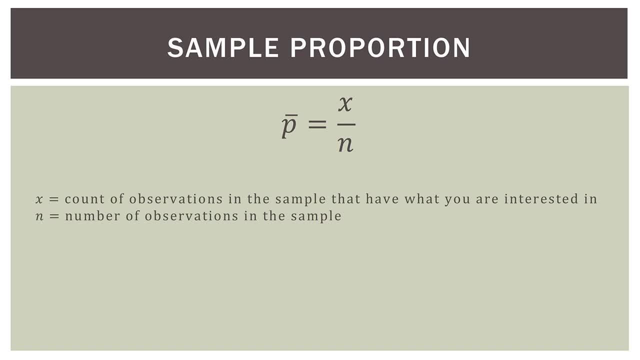 And that equals x over n, where x is the count of the observations in the sample that have what you are interested in. So in this case, it's who answers yes, N is the number of observations in the sample which, again in this case, is 30.. 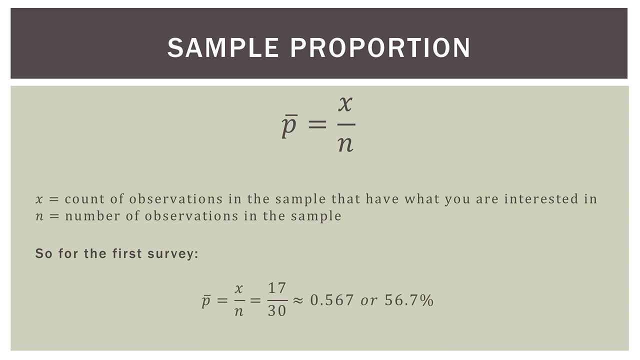 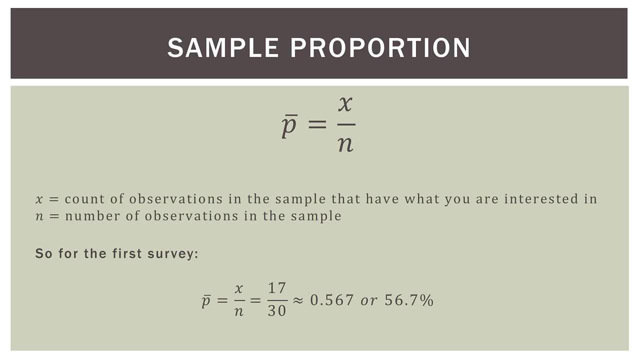 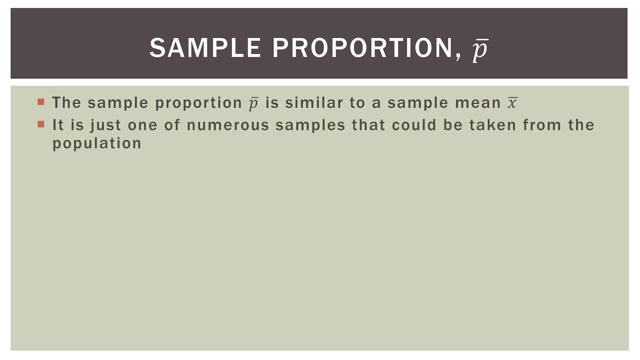 is similar to a sample mean, which was x bar. It is just one of numerous samples that could be taken from the overall population, So in this case the population is the entire student body of Caffeine State University. Now, if someone else went out and did the survey again, 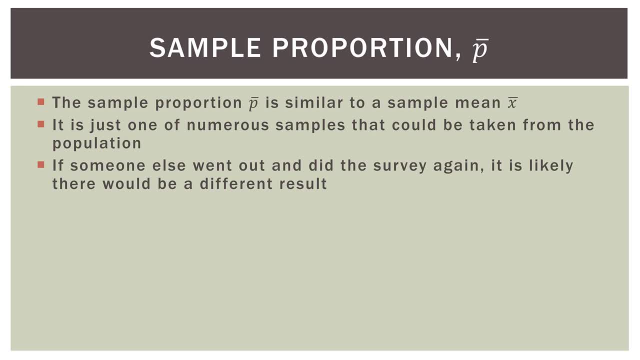 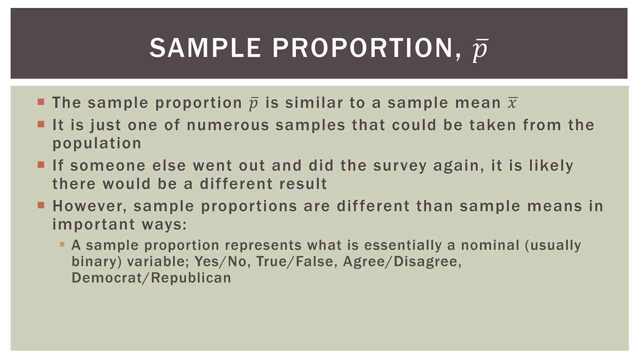 it's likely there would be a different result, just like we did for sample means. However, sample proportions are different than sample means in important ways, So a sample proportion represents what is essentially a nominal, so usually a binary, variable, So something like yes, no, true, false. 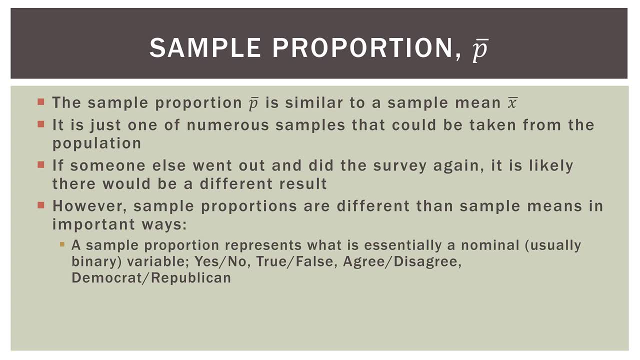 agree, disagree and, like elections, could be Democrat, Republican, et cetera. So usually it's binary, meaning two options, and they are exclusive, So you can't be yes and a no or something like that. So it is a count or frequency. 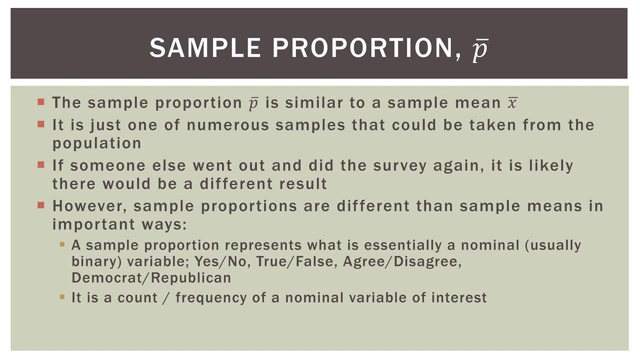 of a nominal variable of interest. Now I will say at this point: there are proportions that have more than two options And you can compare those proportions and we'll get to that eventually, But for the sake of this video we're gonna stick to two options. 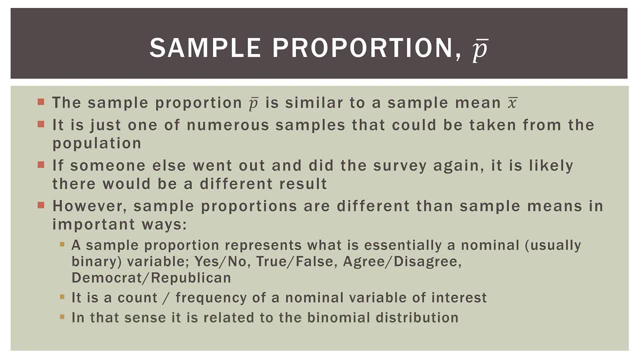 a binary choice of yes, no, true, false, et cetera. So in that sense it is related to the binomial distribution. I don't wanna get into the weeds here, but if you remember there's a specific distribution. 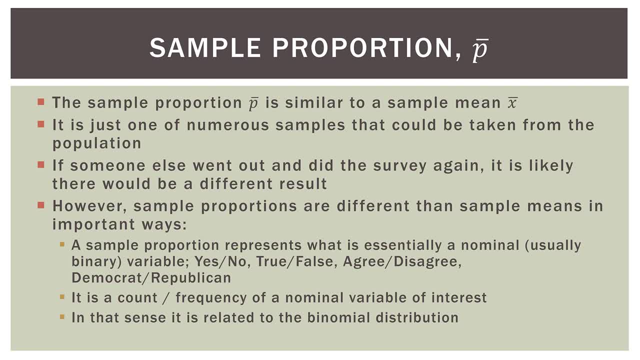 called the binomial distribution, where we talk about successes and failures, where we have two options. So the sample proportion is somewhat related to that and you might see some similarities as we go forward. For the sake of just learning this concept, it's not overly important. 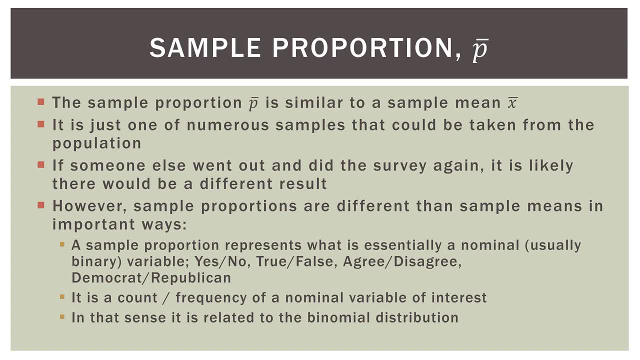 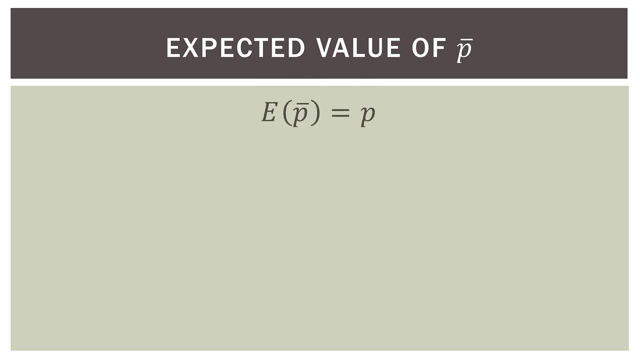 but I just wanted to point out that it is similar to the binomial. So what is the expected value of P bar? the sample proportion? So the expected value equals P, which is the population proportion. So the expected value of the sample proportion, P bar. 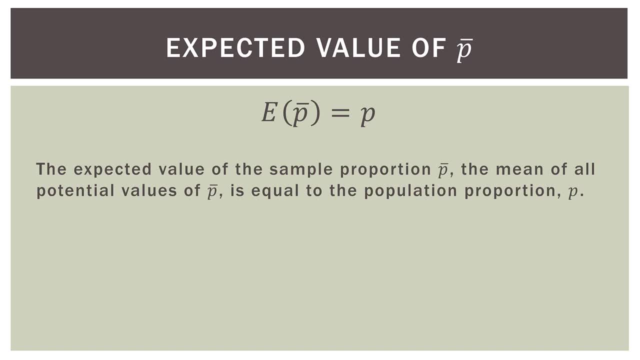 the mean of all potential values of P bar is equal to the population proportion P. So another way of saying that is that if we went out and took many sample proportions from the same population over and over, and over and over again, the mean of all those sample proportions 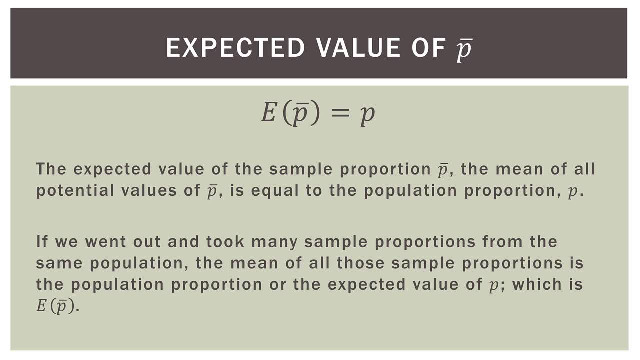 is the population proportion or the expected value. So the expected value is equal to the mean of all those sample proportions E of P bar. So the way to think about this is that the expected value of the population proportion is just taking many. 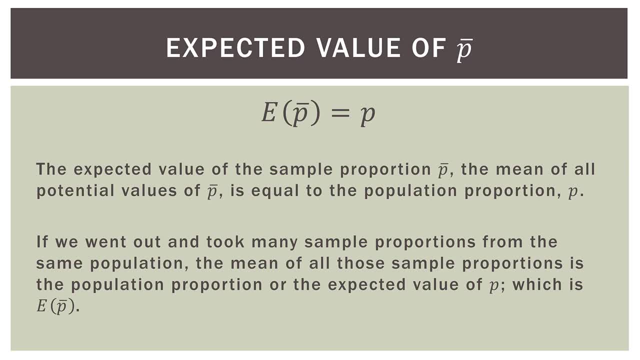 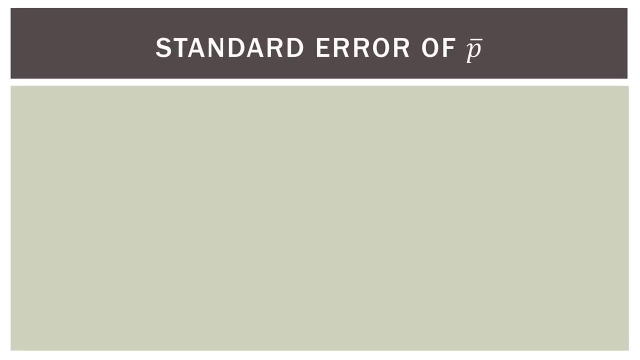 many samples and finding the mean of all those sample proportions. That's the expected value. So if we went out and took many sample proportions over and, over and over again and we collected all of those sample proportions, we put those into its own distribution. 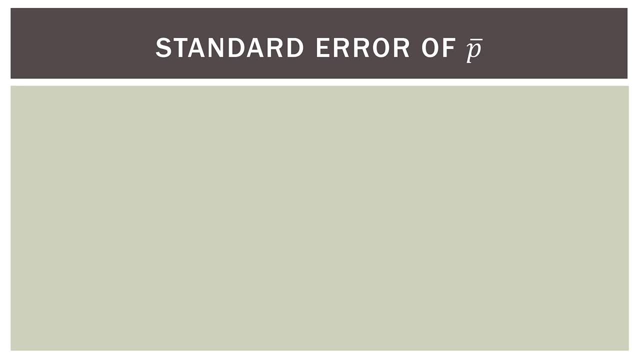 is a sampling distribution. If you remember from the previous videos, we talked about the sampling distribution for the mean Now, any distribution like that is gonna have its own standard deviation and the name of that is called the standard error. So the standard error is the standard deviation. 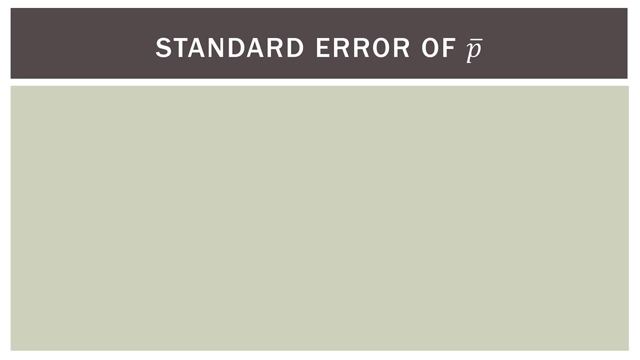 of a sampling distribution and that goes for sample means or sample proportions. So we refer to the standard deviation of the sample proportion as the standard error of the sample proportion. However, the standard error of p-bar, our sample proportion, is dependent on a question. 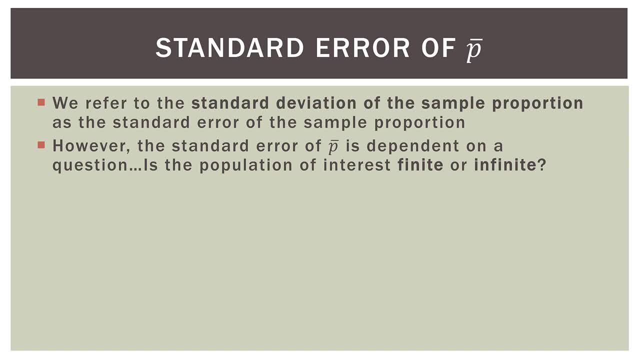 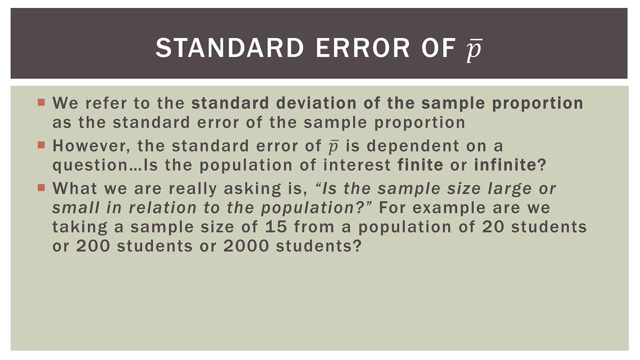 and this is unique to sampling proportions, not sample means. Is the population of interest finite or infinite? So what we're really asking is: is the sample size large or small in relation to the population? For example, are we taking a sample of 15? 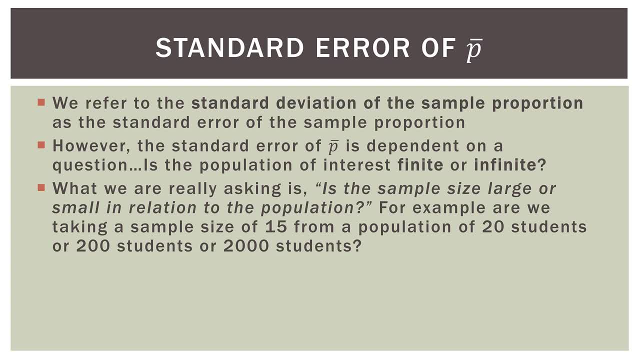 from a population of 20 students, like maybe just one classroom, or 200 students like a very large lecture, or 15 from 2,000 students, maybe a small college. So we're looking for the relationship between our sample size and the overall population. 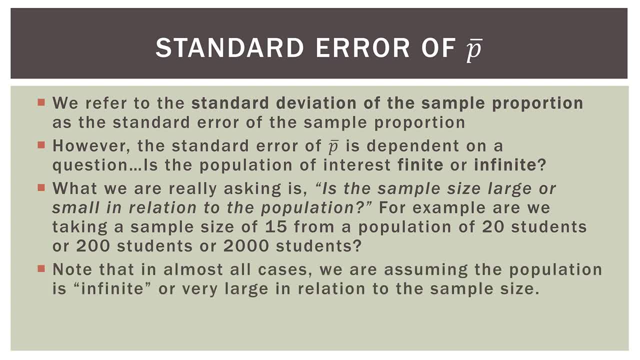 that we're interested in and we have to ask this question Now. note that in almost all cases in practice- like in your class or whatever else we are assuming- the population is infinite or very large or large enough in relation to the sample size. 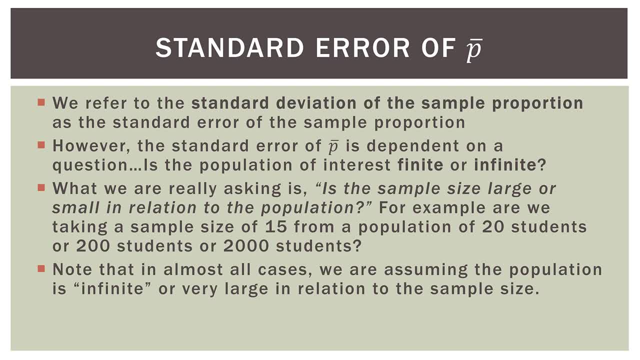 Probably not something you're gonna have to worry about doing your homework or something else like that, because we kind of assume that the sample size is small relative to the overall population. but we just have to ask ourselves that question or at least note if it's out of the ordinary. 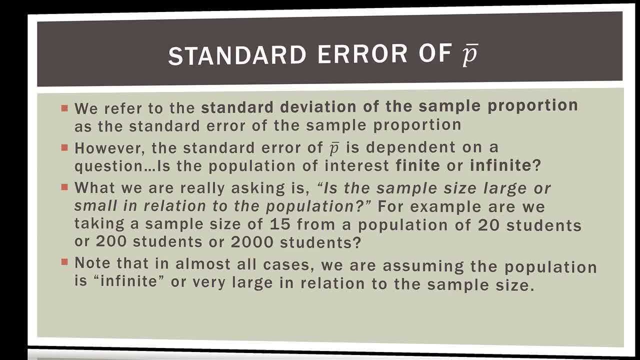 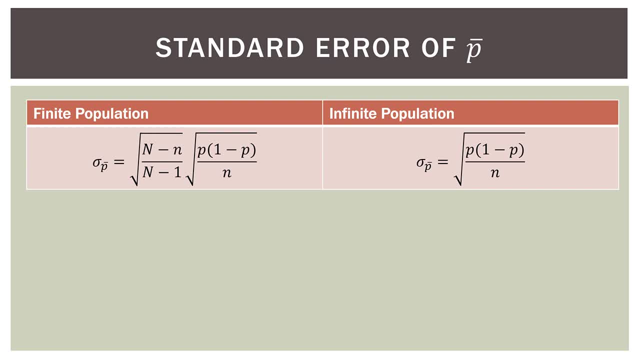 because we're taking it from a very small population. So, depending on the answer to that question, we have a slightly different standard error. So the standard error is sigma sub p-bar And again, remember, for sample means it's sigma sub x-bar. 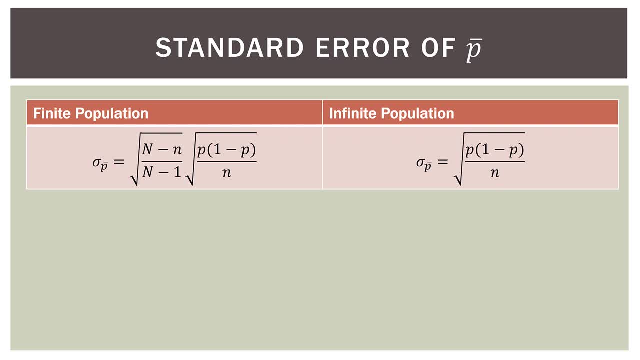 Same notation, very similar. So on the left we have the standard error if we're taking it from a finite population, and on the right we have the standard error if we're taking it on a infinite population. They're very similar except for the one expression. 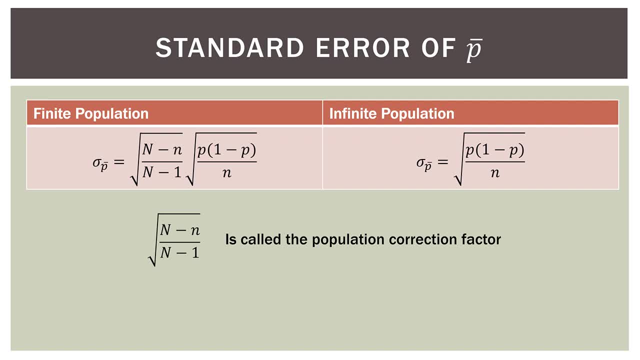 there at the beginning. So that is called the population correction factor. We only employ that if we're taking a sample from a population that's small relative to our sample. So the general rule is that if small n the sample size, over big N the population size. 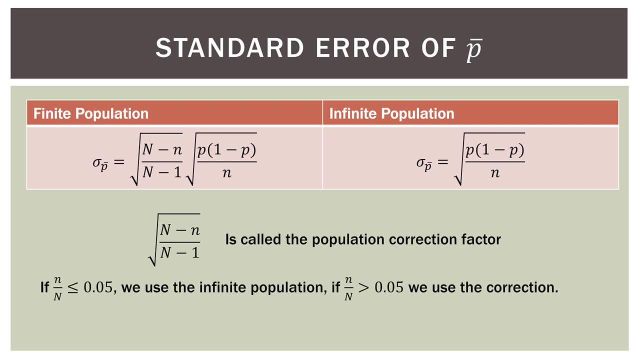 is less than or equal to .05, we use the infinite population. Now if small n over large N is greater than .05, we have to use that correction factor. So again, in practice, this is probably something you'll never have to encounter. 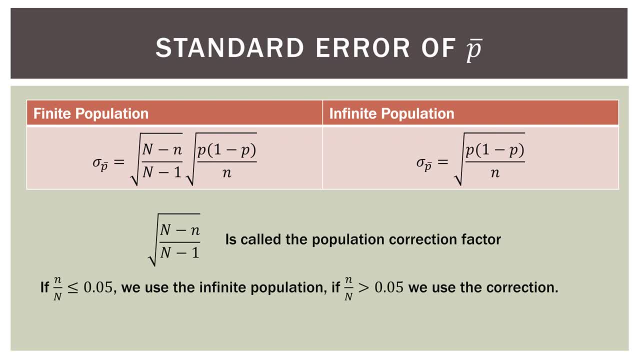 but if you're doing small samples and small population work, then you'll have to keep this in mind. So, for example, we're sampling 30 students on a large college campus, So we're definitely going to use the infinite population standard error. 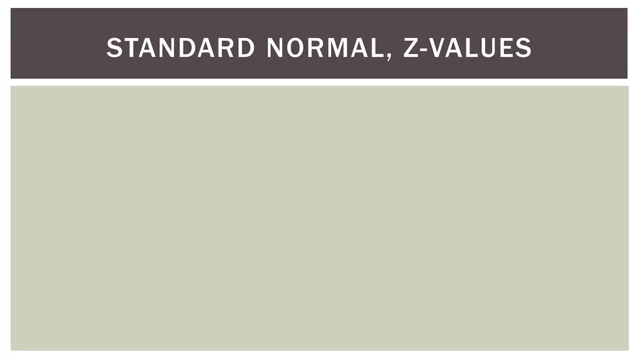 over here on the right. So if our sampling distribution of sample proportions is approximately normal, we can go ahead and find z values like we did in sample means. So we do that, the exact same way To find a z value. we take the sample proportion. 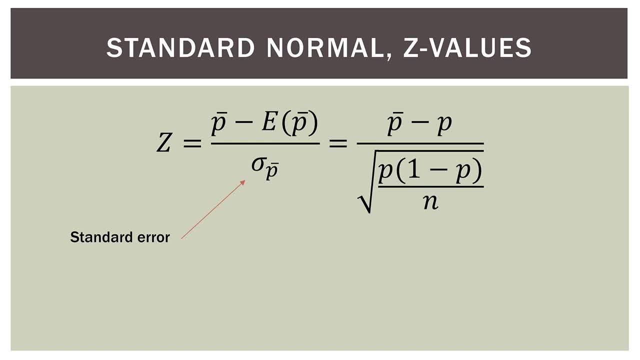 in this case p bar minus p, which is the population proportion divided by the standard error. And when we extract everything out and substitute, we have the expression over here on the right. So this is the same basic form as the sample mean. 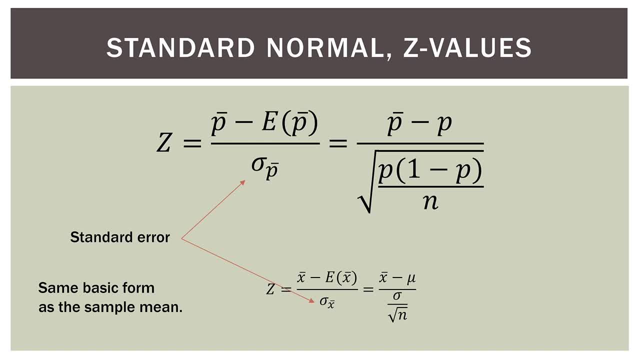 So remember to find a z value, we took x bar, which is the sample mean minus mu, which is the population mean divided by the standard error, which in that case was sigma, divided by the square root of n. So if you look at these two, they're very similar. 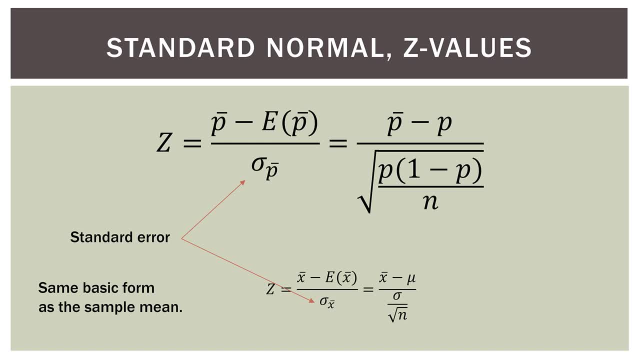 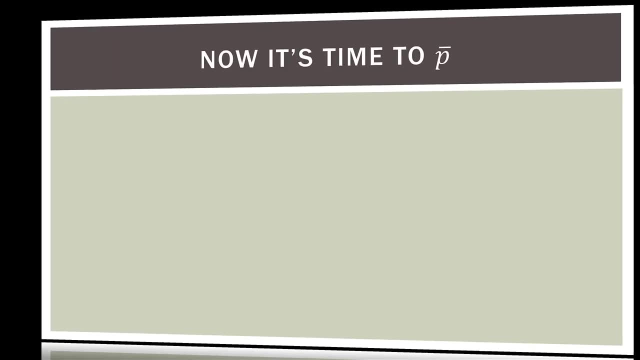 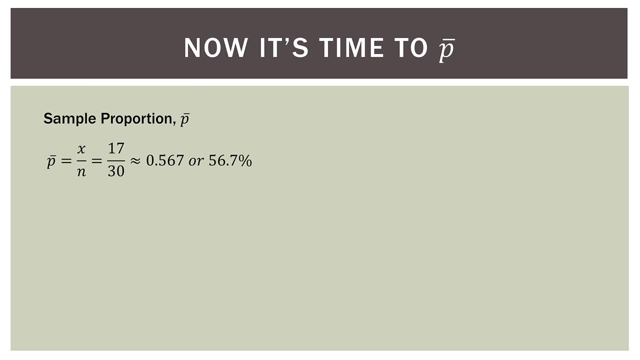 So we have the difference between the sample and the population divided by the standard error in each case. so the same basic form. So now it's time to p bar. So here's our sample proportion. So remember that was 17 divided by 30,. 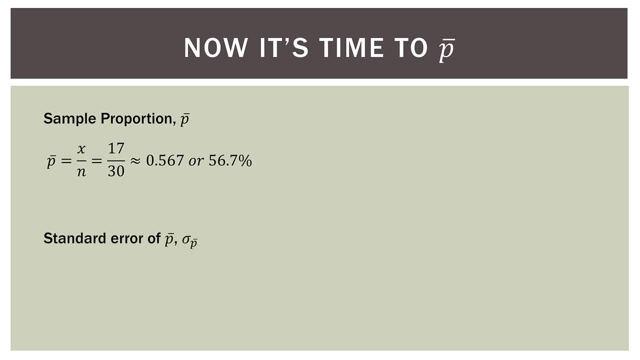 or 0.567.. So now we can calculate the standard error using our formula. down here We substitute everything in, So for p we have 0.567, and then one minus that. We multiply those together, divide by n, which is 30,. 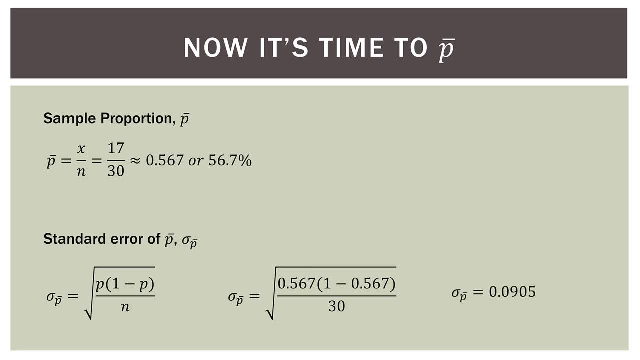 and then take the square root of all that and we have 0.0905.. So the standard error of p bar, our sample proportion, is 0.0905.. 0.0905.. So before we go any further, we have to run two tests. 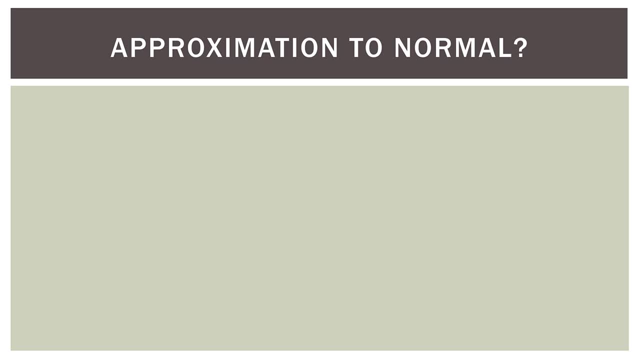 And again in normal, you know class or homework problems you're having. you probably won't have to do this. You might, but I'm just gonna mention it because I would be derelict if I did not. So we have to make sure that we can use 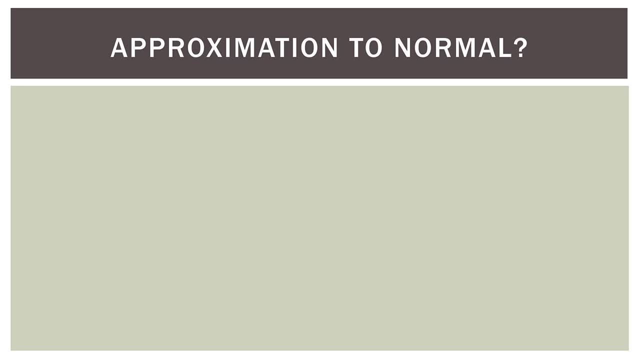 the normal distribution for our sampling distribution. in this case- and it's very simple to do- We gotta run two quick tests. So the first is n times p greater than or equal to five. We're evaluating this as true or false. So we do that, math out. 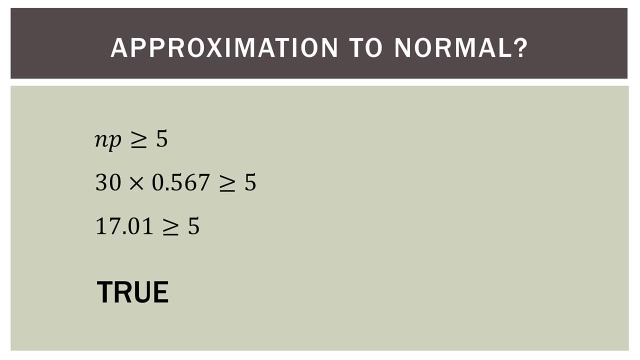 We end up with 17.01.. That is greater than or equal to five. so that is true. Then we do the other side. So we do that math and we end up with 12.99.. That is greater than or equal to five. 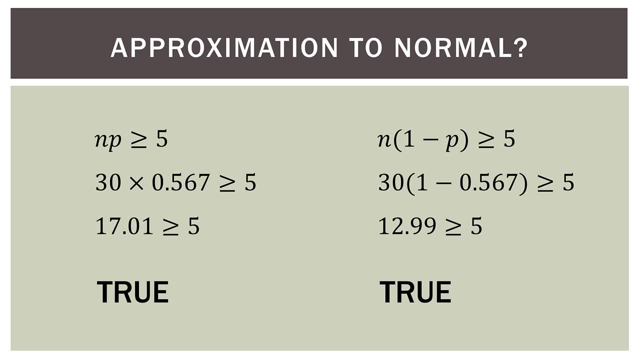 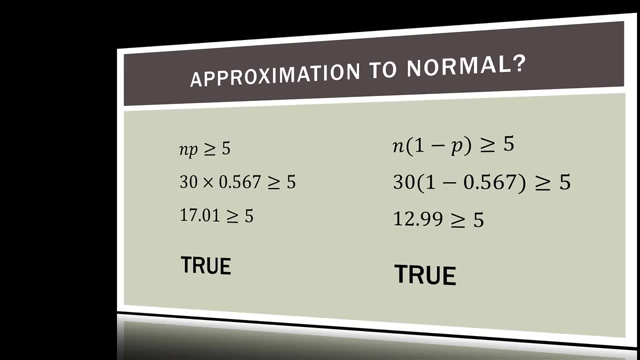 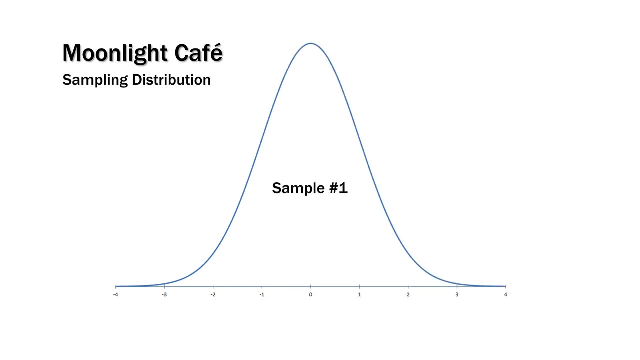 That is also true. So as long as those are both true, we can use the normal distribution as an approximation of our sampling distribution for the sample proportion. And here it is. So once we pass the two tests in the previous slide, we can go ahead and use this normal distribution. 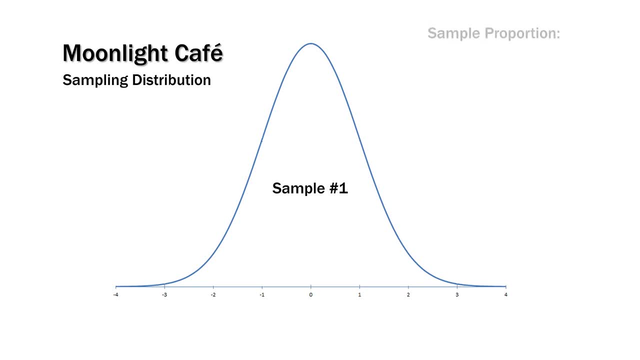 to represent our sampling distribution for the sample proportion. So our sample proportion was 0.567.. So we take that and we center that in our sampling distribution right here in the middle. Remember that is a z value of zero, right here in the middle. 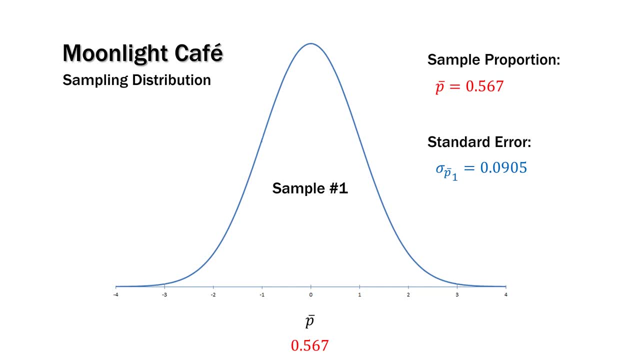 Our standard error is 0.567.. Our standard error is 0.0905.. And what that represents is a z value of one. So we can go ahead and put 0.0905 above one: a z value of one. 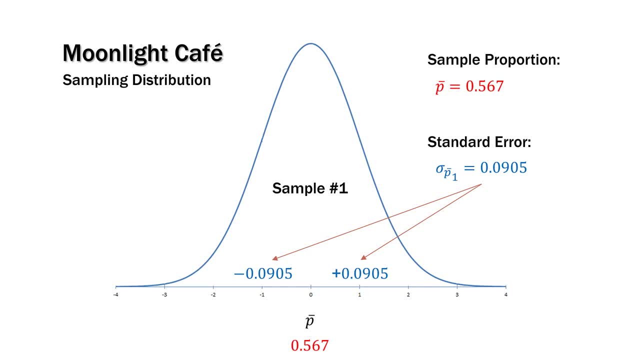 And then the negative of that is a z value of negative one. So think and remember that a z value of one is just another way of measuring the standard error, which is 0.0905.. It's like measuring something in centimeters. 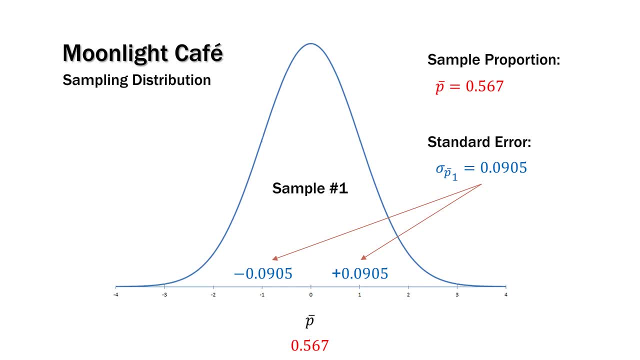 or inches. The distance on paper is the same. You're just measuring it with a different unit. So they're the same distance, just different units. So we go ahead and do the addition and subtraction and now we can place actual values for each z value. 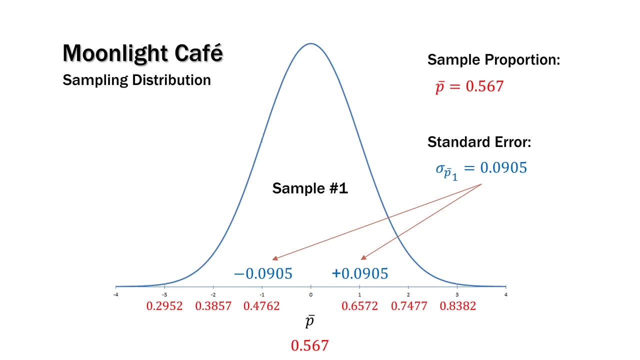 So if you look here at the z value of one, we take 0.567 plus 0.0905, and we end up with 0.6572.. Then we do that again and again to get a z value of two and a z value of three. 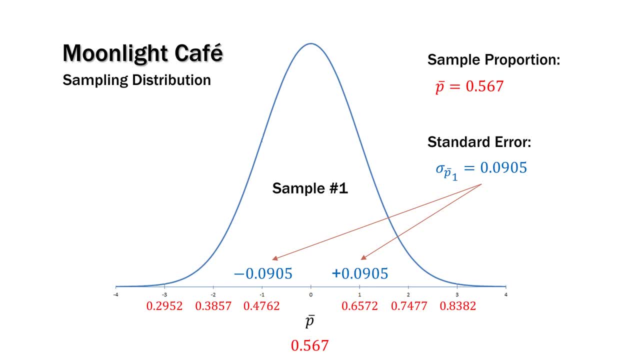 Then we do the other half of the distribution by subtraction, So 0.567 minus 0.0905, we get 0.4762, and then negative two and negative three. So now we have the actual values for our z values. 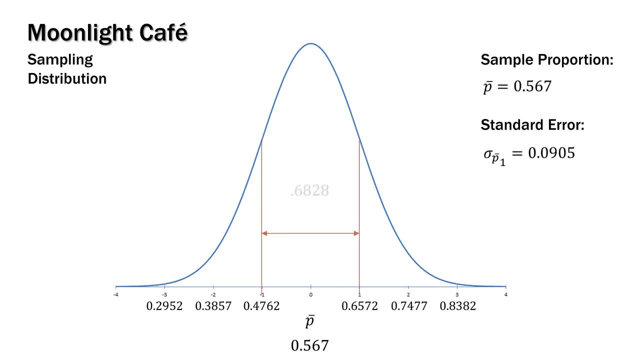 So if you remember something called the empirical rule and that says that about 68% of our sample values are z values, So that means that about 68% of our sample values should be within one standard error or a z score of one from the mean. 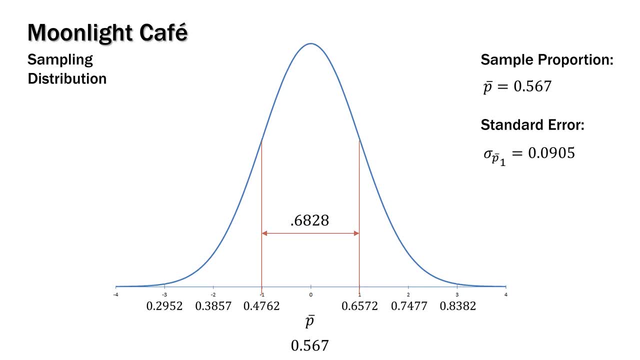 So if we did this over and, over and over again, we would expect about 68% of those values to fall in this interval Now about 95% within two standard errors or a z value of plus or minus two, And about 99% or almost all values. 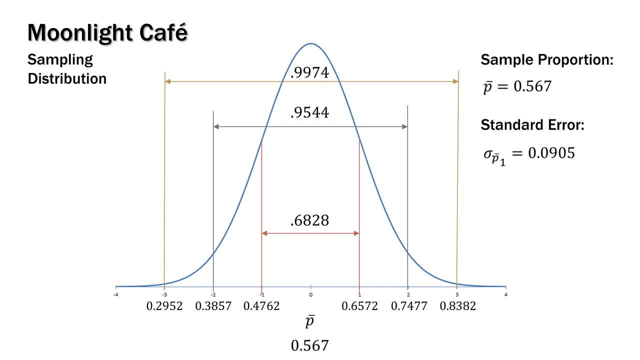 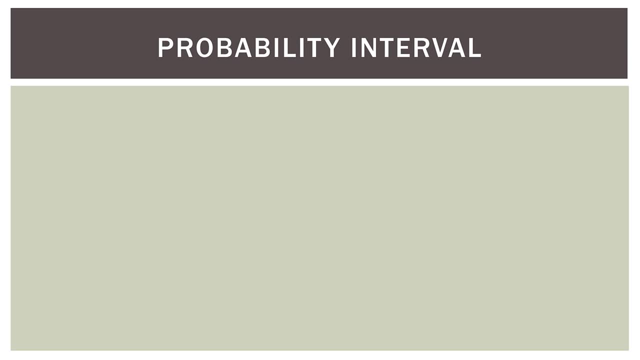 should fall between plus or minus a z value or a z value of three or three standard errors in each direction. So what about a probability interval using that sampling distribution? So the administration would like to know the probability of obtaining a sample proportion that is between 0.55 and 0.65.. 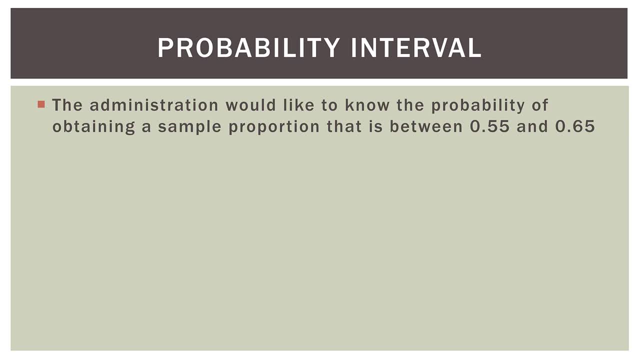 So we're interested in a sliver of that sampling distribution So we can use the sampling distribution to find this probability, just like we did for sample means- Exact same process. So here's what we're looking for: We're looking for the probability. 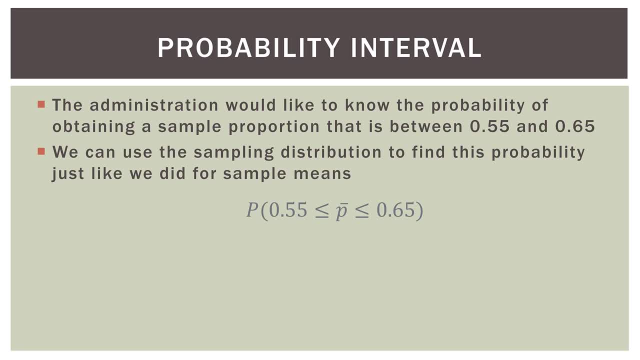 of obtaining a sample proportion that is between 0.55 and 0.65.. So we're looking for a sliver of that distribution. So what we're gonna do is find two probabilities and then subtract one from the other. So the first thing we're gonna do 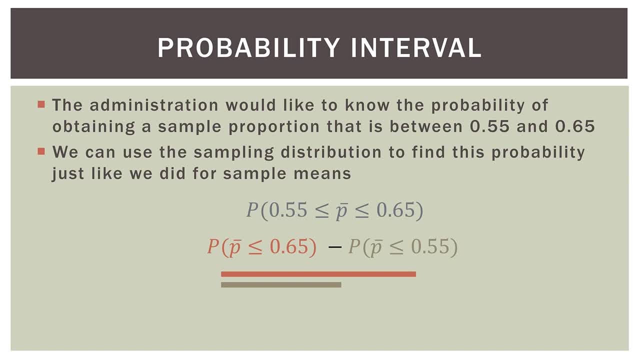 is find the cumulative probability of having a sample proportion of 0.65.. Then we're gonna find the probability- the cumulative probability that is, of a sample proportion of 0.55.. Then what we're gonna do is subtract the smaller one. 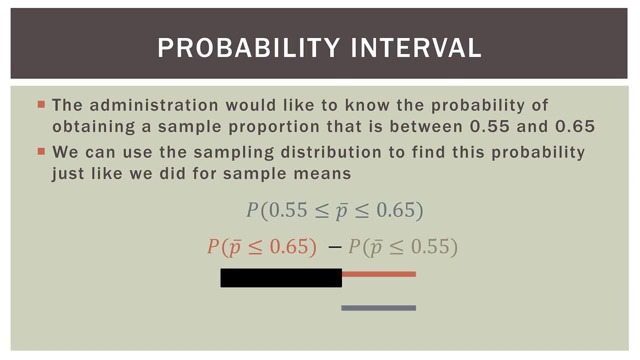 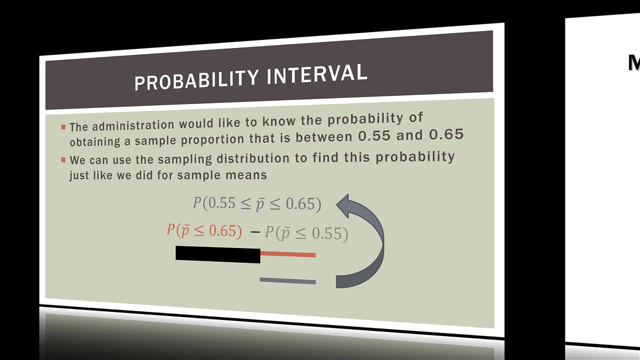 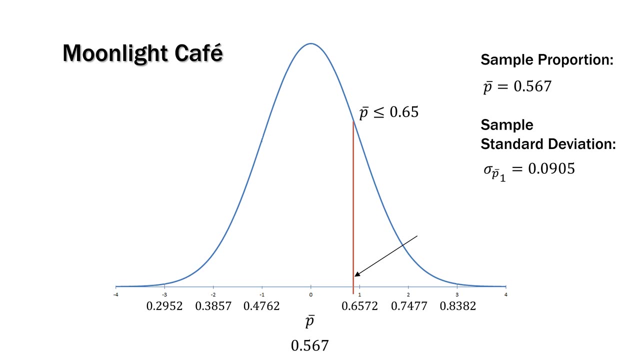 from the larger one and we'll end up with the difference, And that will give us the sliver in the sampling distribution that we are interested in. So visually it looks like this. So here's the upper value we're interested in, So 0.65.. 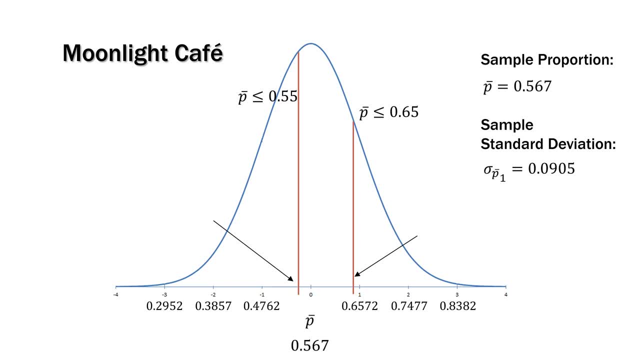 Here's the lower value. we're interested in 0.55.. And you can see how those fall relative to the values along our bottom axis And we're interested in the difference. So we're gonna take everything from the left to the upper value. 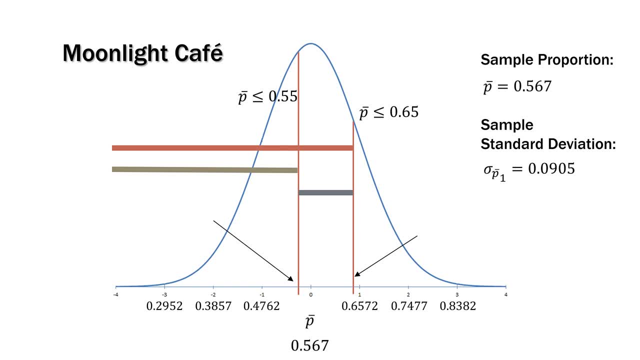 everything from the left to the lower value subtract, and then we're gonna get this gray sliver in the middle, which is what we want. right there, We're looking for the area of that section. So the first thing we have to do 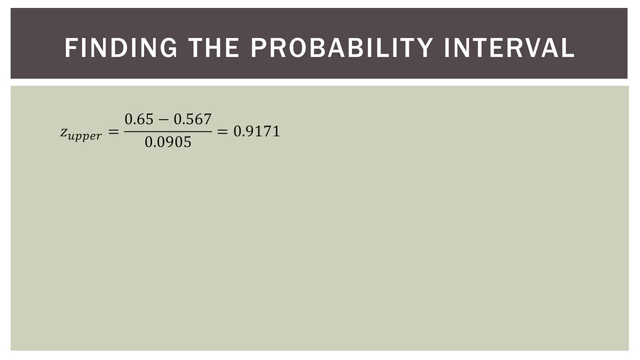 is find the Z value for that upper boundary, And we do that very simply by subtracting the upper boundary 0.65, minus the sample proportion, which is 0.567, divided by the standard error. So what we're asking here is how many standard errors? 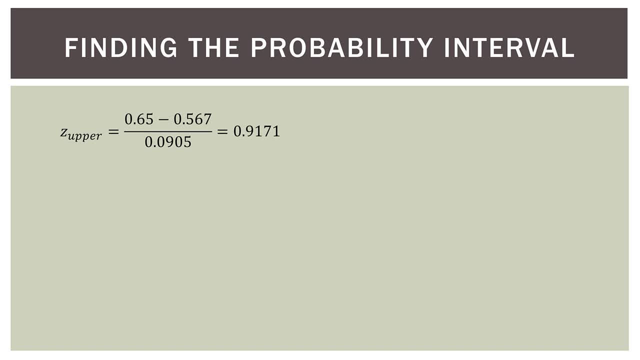 how many standard deviations is 0.65 above the mean. So in this case we do the math and we have 0.9171.. So the sample proportion is 0.9171.. So the sample proportion is 0.9171.. 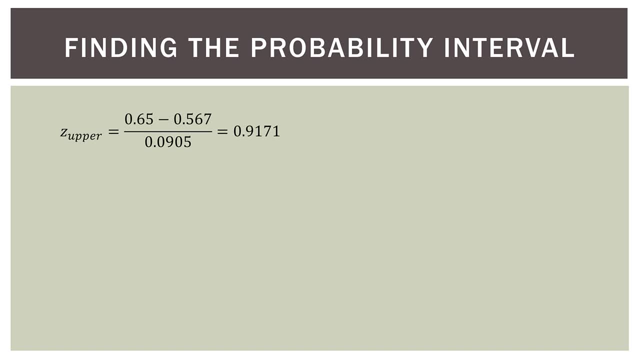 So the sample proportion of 0.65 is 0.9171 standard errors or a Z value of 0.9171.. Same thing with the lower, So 0.55 minus the sample proportion divided by the standard error. 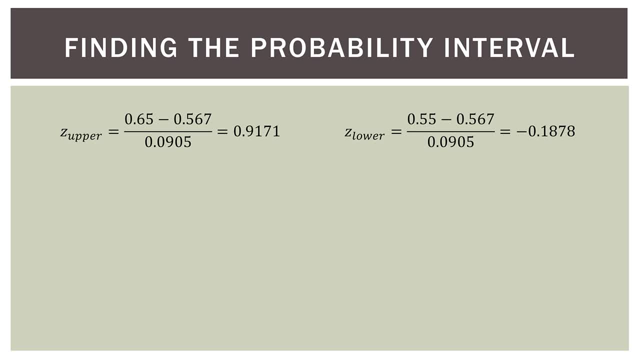 and we end up with negative 0.1878.. So the sample proportion of 0.55 is- you can say it either way- so 0.1878 standard errors below the sample proportion. So again, we just subtract, So we find the probabilities, the cumulative probabilities. 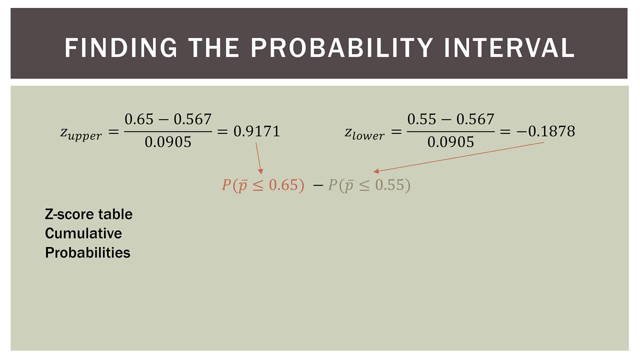 using our Z-score table in the back of the book or online phone app, whatever you have. So the cumulative probability to a Z value of 0.9171, remember that's the longest one that we had in the previous slide- is 0.82.. 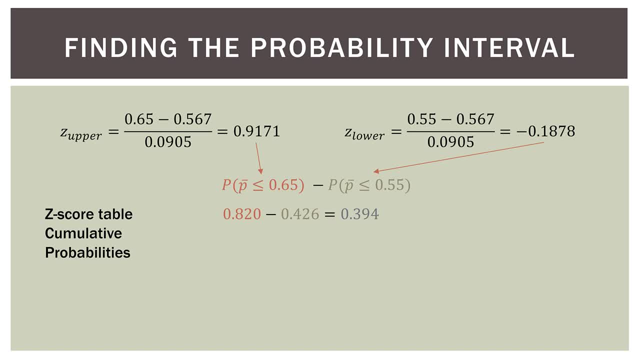 So that represents 82% of the area under that curve. Then we find the cumulative probability left to right of 0.55, a sample proportion of 0.65.. a sample proportion of 0.55.. That is 0.426. 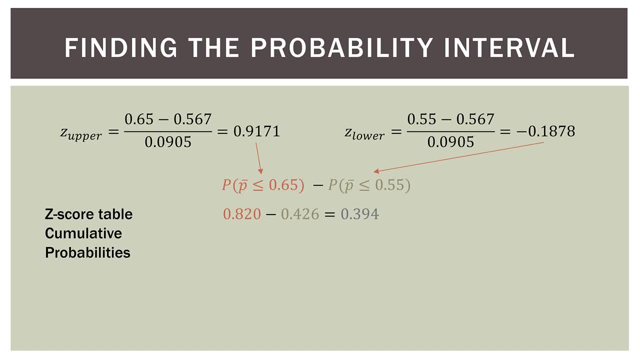 So that's 42.6% of the area under the curve. Then we just subtract out the smaller one and we end up with what we want. So we go ahead and do that and that is 0.394.. So approximately 39.4% of sample proportions. 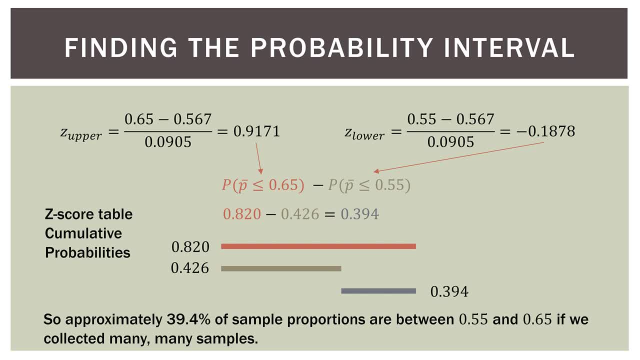 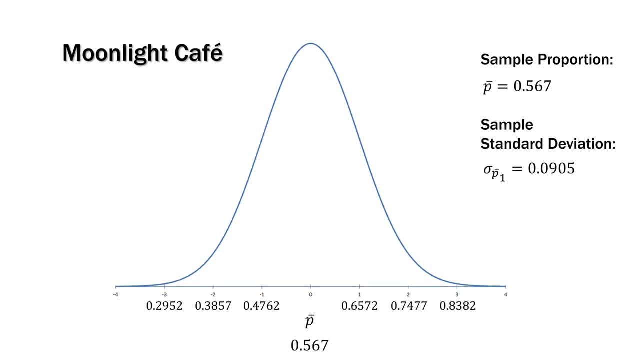 are between 0.55 and 0.65. if we collected many, many samples over and over and over again, It looks like this: So here was our upper boundary, Here was our lower boundary, And that's what we got. So we can expect about 40% of sample proportions. 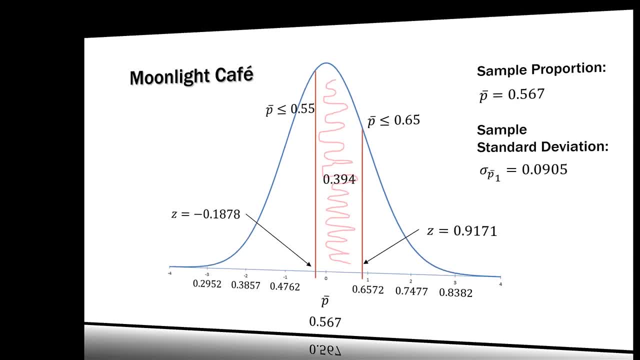 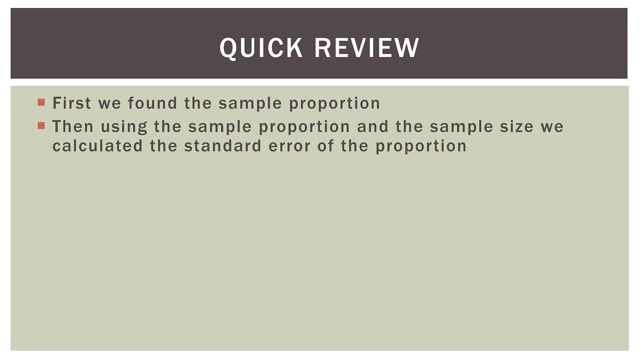 to be in this interval. So quick review: First we found the sample proportion. Then, using the sample proportion and the sample size, we calculated the standard error of the proportion. The standard error of the proportion is the standard deviation of the sampling distribution. 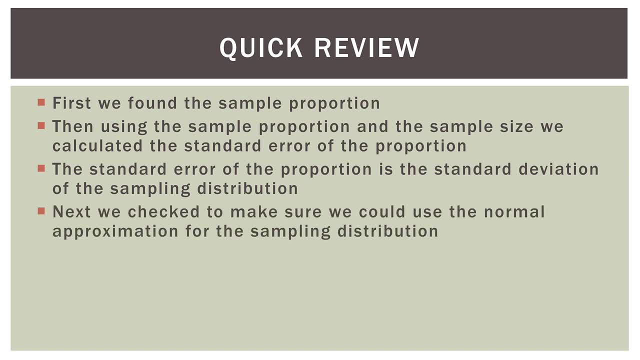 in this case of sample proportions. Next, we checked to make sure we could use the normal approximation for the sampling distribution. Remember that was the two true tests we did on that one slide. If yes, we can go ahead and use the standard error. 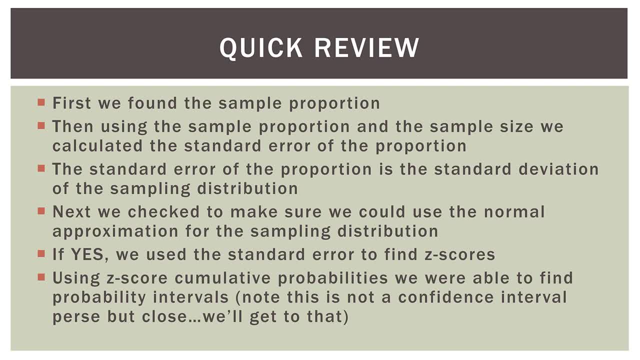 to find z-scores or z-values. So using z-score cumulative probabilities, we were able to find probability intervals. Now I want to note here that you've heard the word interval before, So what we're doing here is not a confidence interval per se. 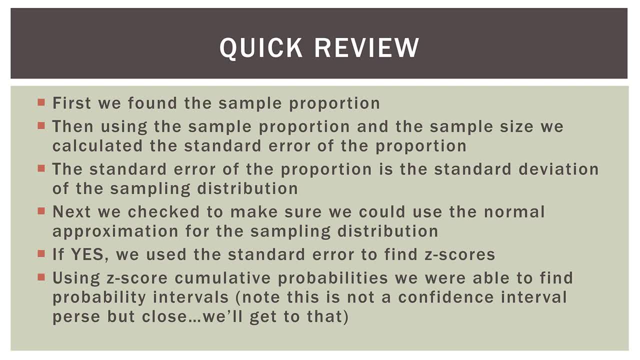 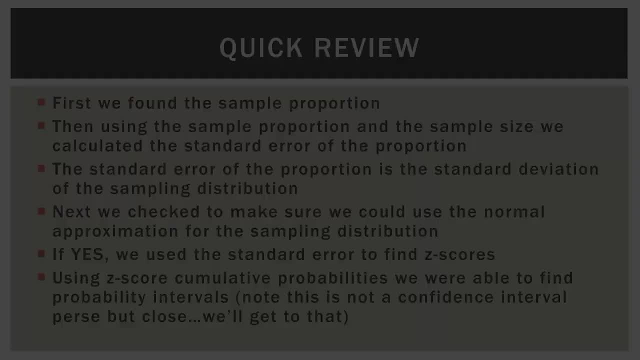 We'll get to that. So all we're doing here is finding slices of the sampling distribution, Okay, and we can do that for any two values. So confidence intervals we'll get to later. This video is brought to you by The Great Courses Plus. 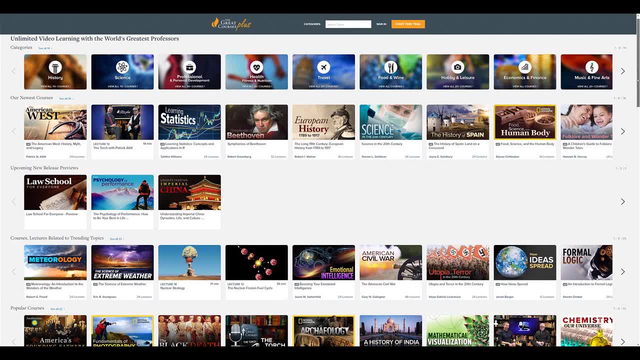 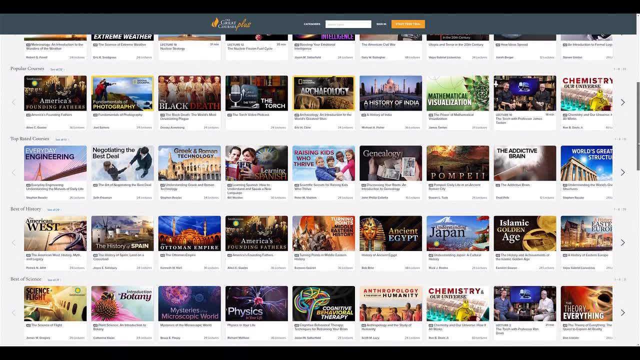 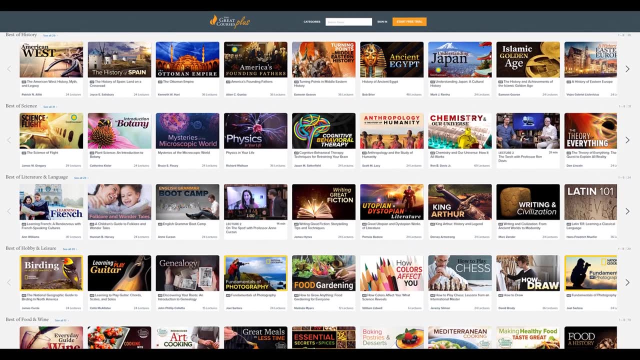 where you can get unlimited access to over 11,000 video lectures taught by award-winning professors from the Ivy League- other top schools around the world. You can learn about anything that interests you: science, literature, photography, gardening and, yes, statistics, like this lecture from Professor Tim Chartier called Got Data. 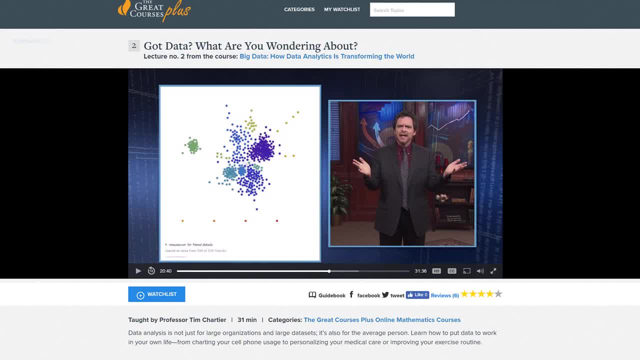 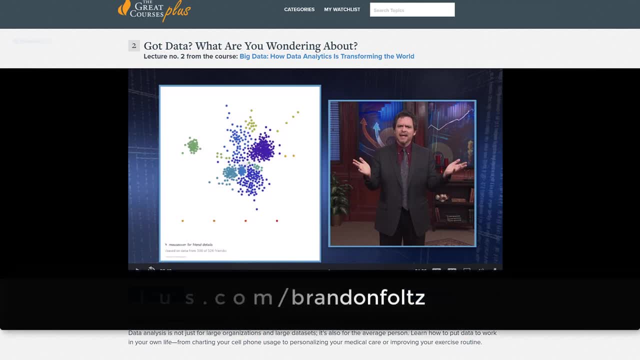 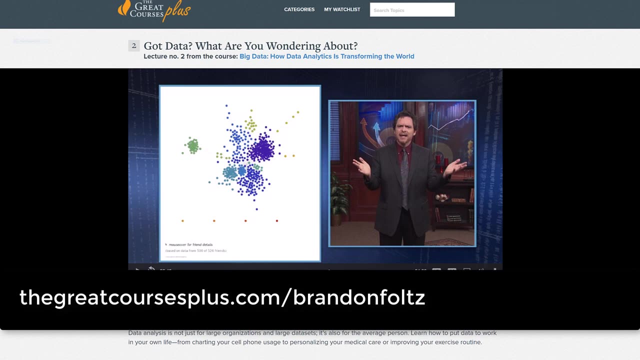 What Are You Wondering About from his course Big Data, How Data Analytics is Transforming the World. And right now, The Great Courses Plus is offering my viewers a free trial and is also now optimized for Australia and the UK. So go to thegreatcoursespluscom, slash Brandon Foltz, my name- to have access to the over. 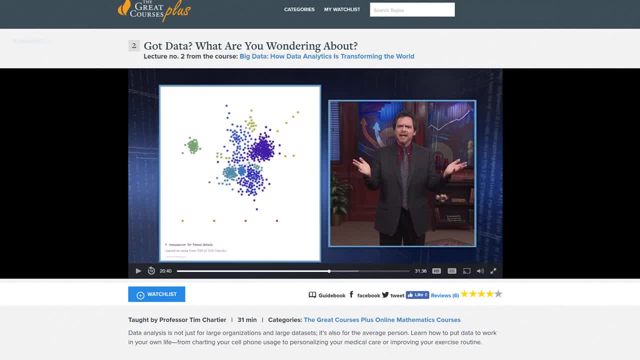 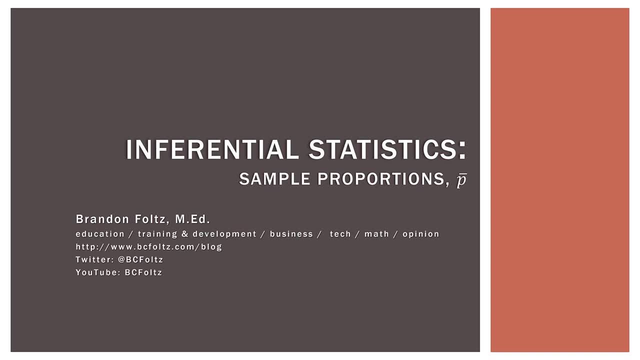 11,000 video lecture library or click on the link in the description below. Okay, so that wraps up this video on an introduction to sample proportions. Again, many of the things we saw in this was very similar to sample means. It's a different kind of data, but when we found the standard error and everything, the 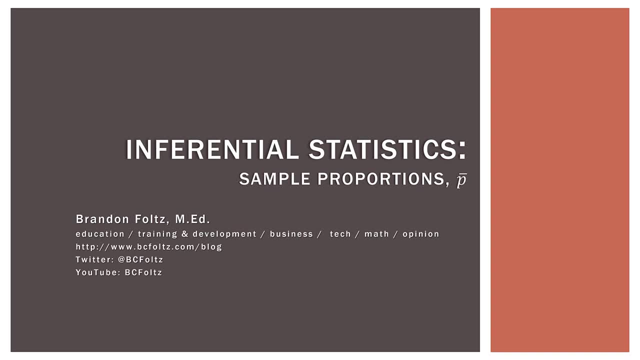 forms of those were similar. When we found the Z values in the sampling distribution, that was great, That was all the same. So there are a lot of things you can carry over from sample means to sample proportions. So anyway, I hope you liked the video. 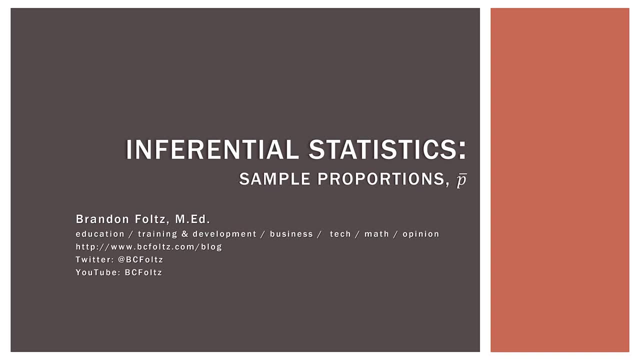 Again. if you like it, please give it a thumbs up, share it with anyone you think might benefit from watching, and thank you for your time and I look forward to seeing you again in our next video. Goodbye. 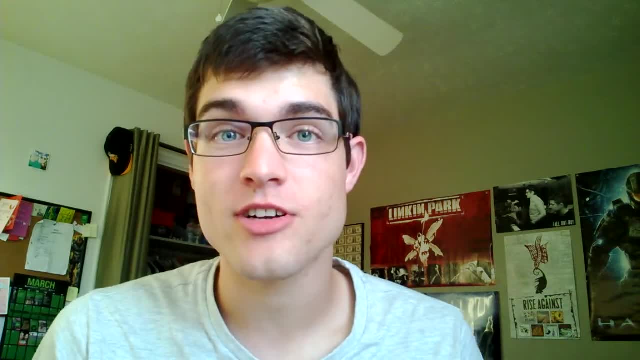 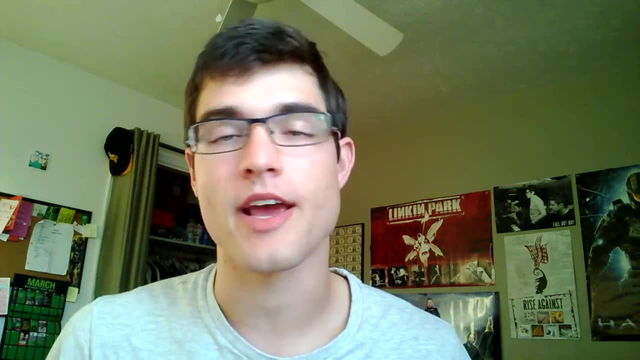 Hi, my name is Cal Fletcher and I am a mechanical engineering technology major. The reason I decided to be an engineering technology major is that I've always been interested in mechanical systems. you know the way they work in real world products, whether it be like planes or cars, or just motors themselves. 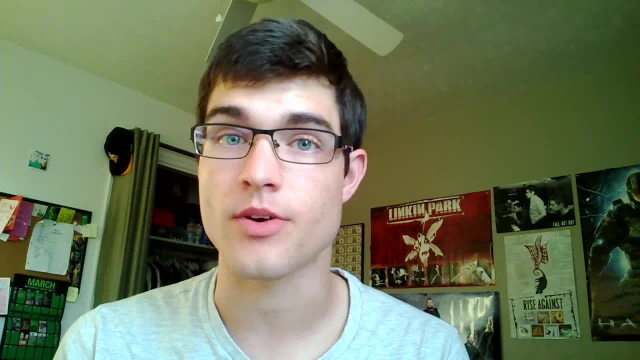 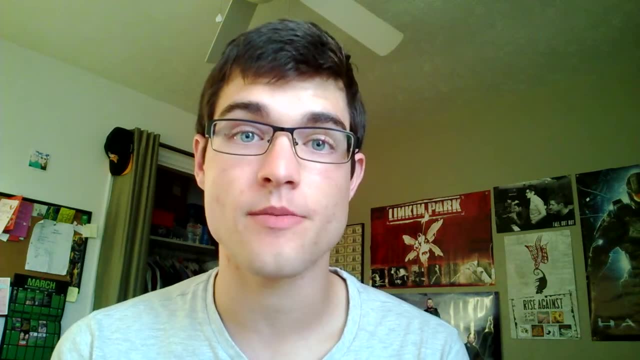 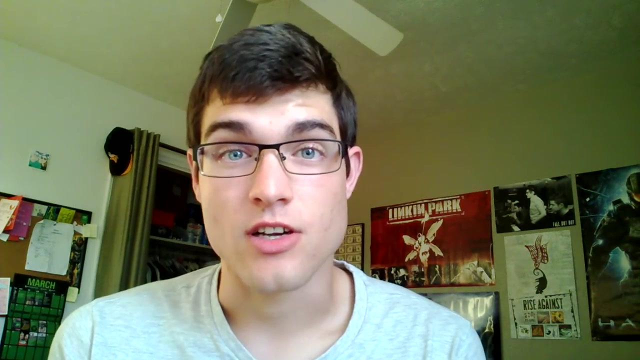 how they work within each other and work in real world products. I've always liked that and been interested in being able to make and design things that people use in actual life or day to day basis. The difference between someone who is in mechanical and energy engineering versus engineering technology. 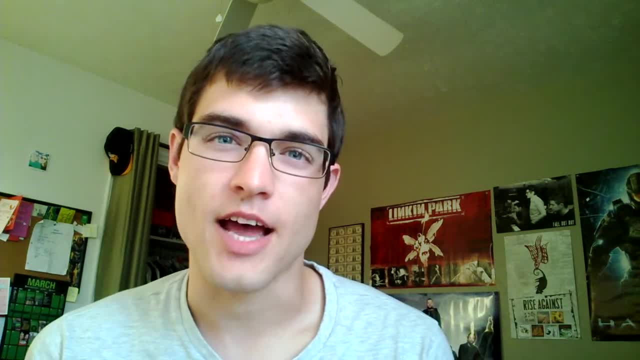 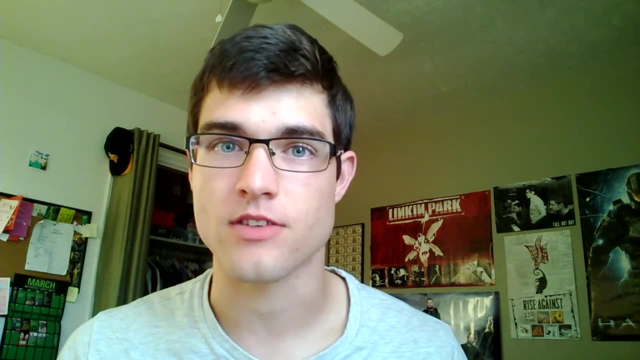 is, the people who are doing energy engineering are more behind, like the design process of something rather than the actual production of it. So they do like the design work and drawing up the schematics of something And the technology major will take that and actually make the product do the design tests on it. 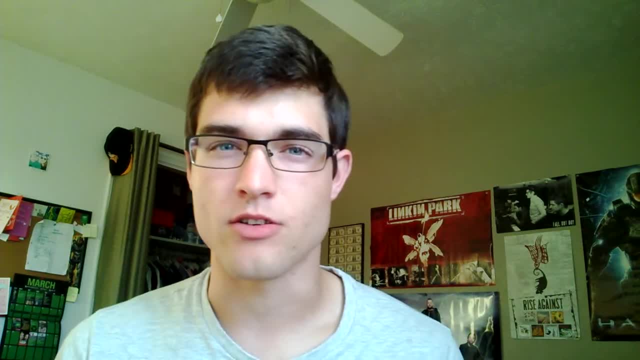 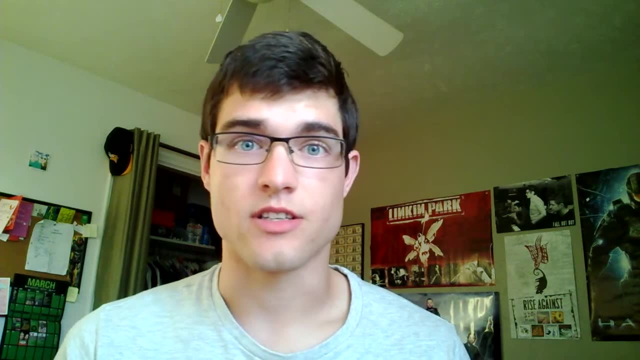 you know my report of what's right and wrong with it. you know send it back And they do more of the hands on stuff with the building of a product, So I've always liked that better, because I can actually physically touch it and mess with it and you know work with it. 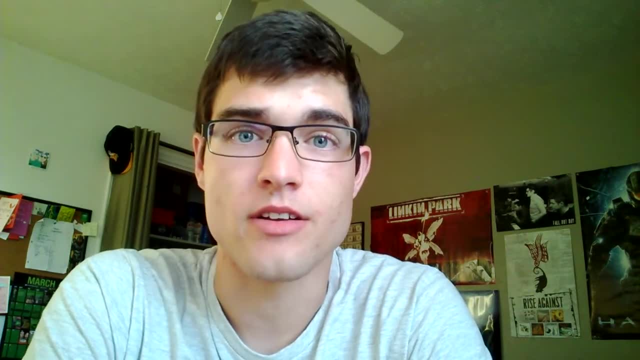 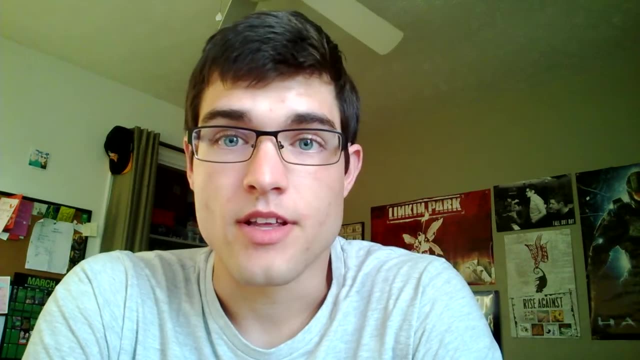 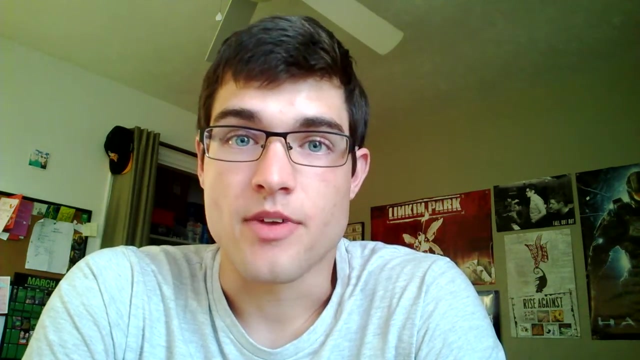 Also the job market difference between a mechanical and energy engineer and an engineering technology major are almost identical. So you know it's pretty good for the employers who will recognize both as very qualified engineers. And I'd rather be in something that I can move forward physically work on than you know do the design of. 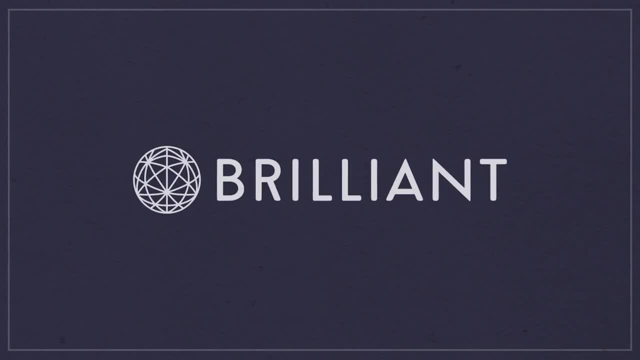 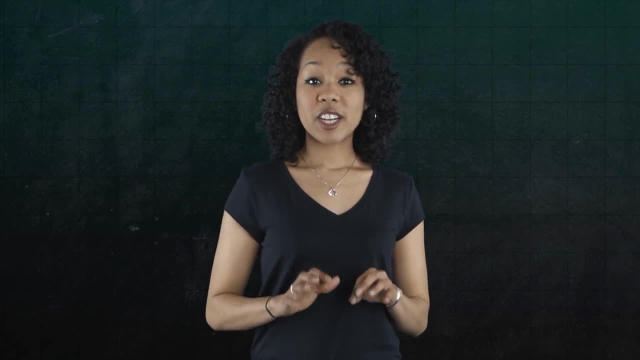 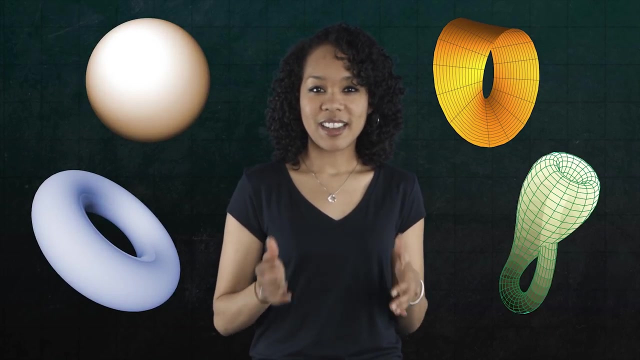 Thanks to Brilliantorg for supporting PBS Digital Studios. We've talked about topology here on Infinite Series. It's the branch of math where we study properties of shapes that are preserved no matter how you bend, twist, stretch or deform them, And you've probably come across some cool examples of these shapes or topological spaces, like spheres and tori, mobius bands and Klein bottles.